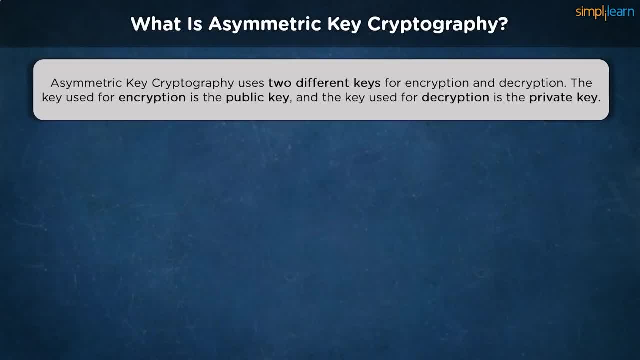 Asymmetric encryption uses a double layer of protection. There are two different keys at play here, A private key and a public key. A public key is used to encrypt the information pre-transit, and a private key is used to decrypt the data post-transit. These pair of keys must belong. 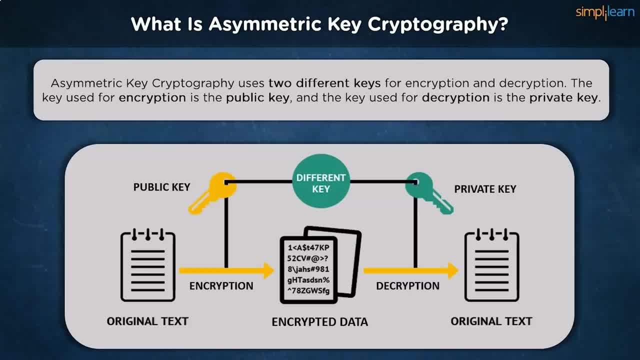 to the receiver of the message. The public keys can be shared via messaging, blog posts or key servers, and there are no restrictions. As you can see in the image, the two keys are working in the system. The sender first encrypts the message using the receiver's private key, after which we receive the cipher. 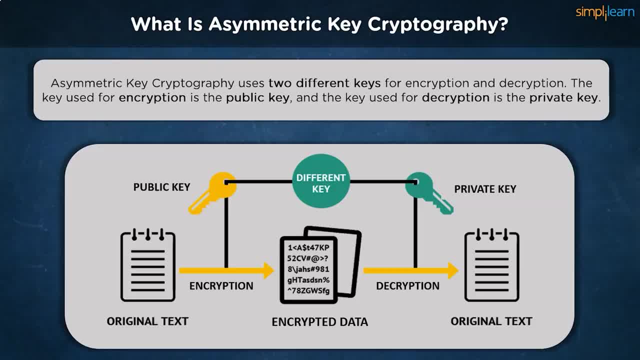 text. The cipher text is then transferred to the receiver. On getting the cipher text, the receiver uses his private key to decrypt it and get the plain text back. There has been no requirement of any key exchange throughout this process, therefore solving the most glaring flaw faced in symmetric key cryptography. 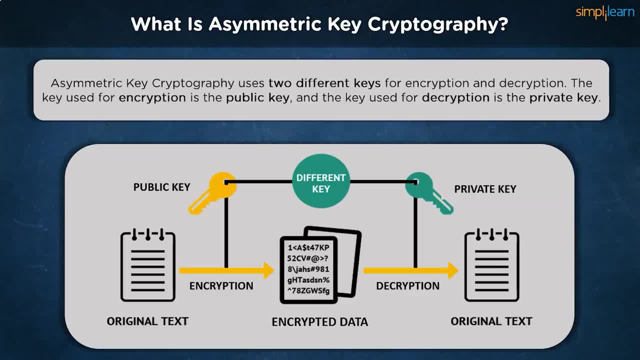 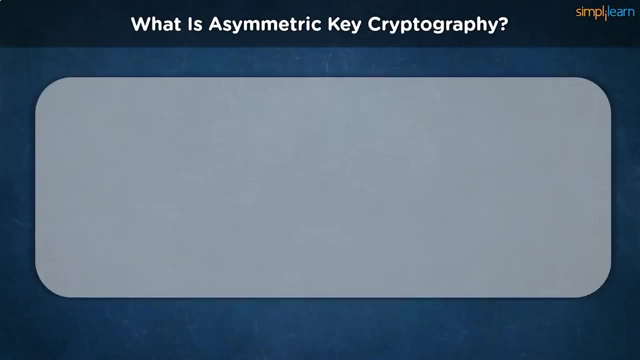 The public key known to everyone, cannot be used to decrypt the message, and the private key, which can decrypt the message, need not be shared with anyone. The sender and receiver can exchange personal data using the same set of keys as often as possible. To understand this better, take the analogy of your mailbox. Anyone who wants to send. 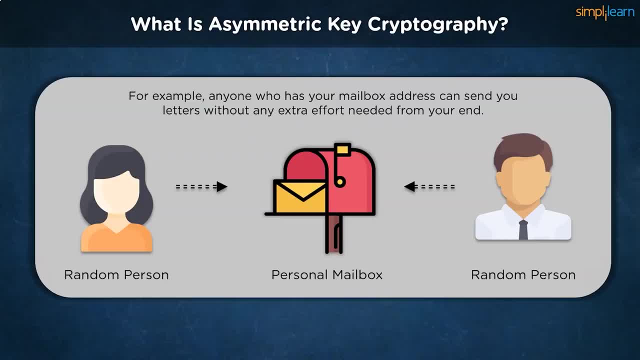 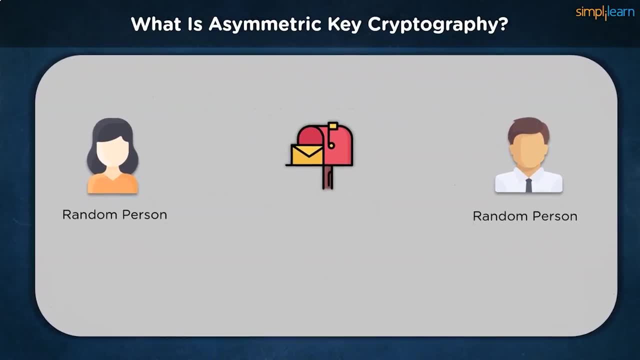 you a letter, has access to the box and can easily share information with you. In a way, you can say the mailbox is publicly available to all, but only you have access to the key that can open the mailbox and read the letters in it. This is how the private key comes to. 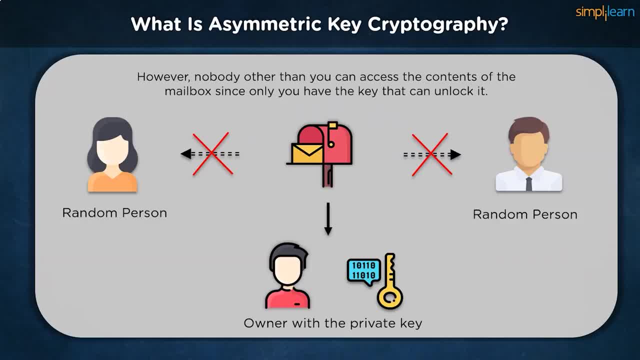 play. No one can intercept the message and read its contents, since it's encrypted. Once the receiver gets its contents, he can use his private key to decrypt the information. Both the public key and the private key are generated so they are interlinked and you 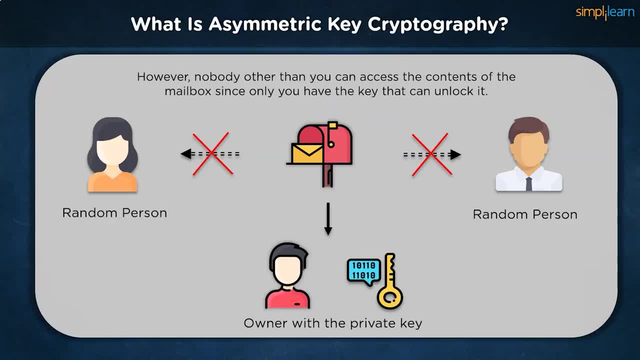 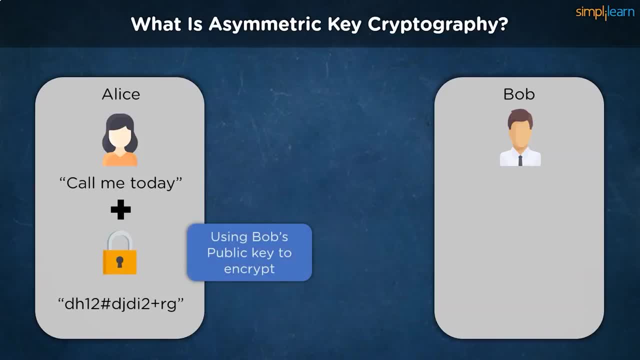 cannot substitute other private keys to decrypt the data. In another example, if Alice wants to send a message to Bob- let's say it reads: call me today- she must use Bob's public key while encrypting the message. Upon receiving the cipher message, Bob can proceed to use his private key in order to decrypt the message. 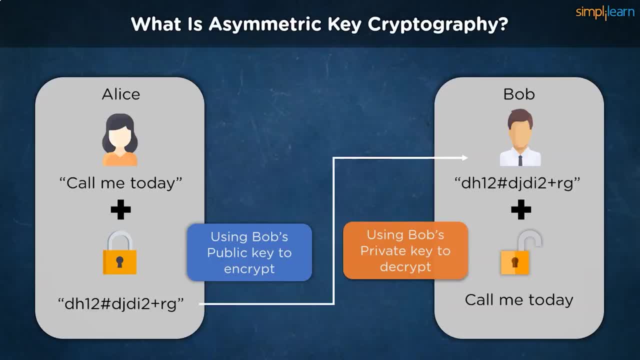 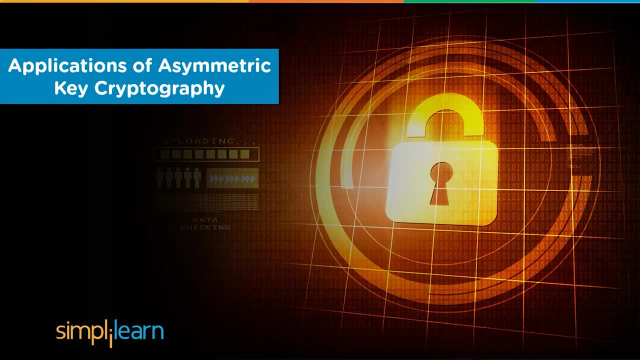 and hence complete security is restored. It's not possible to keep the private key in a safe state for a long time, in case a attained during transmission, without any need for sharing the key. Since this type of encryption is highly secure, it has many uses in areas that require high 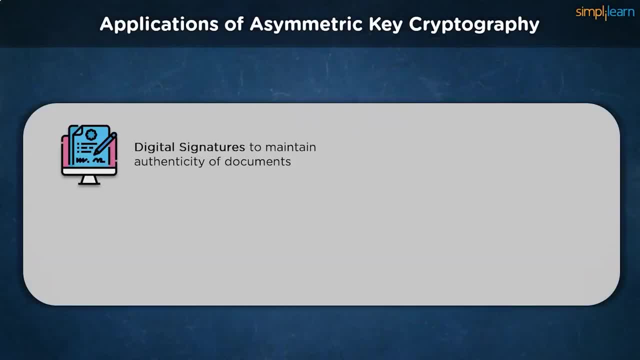 confidentiality. It is used to manage digital signatures, so there is valid proof of a document's authenticity. With so many aspects of business transitioning to the digital sphere, critical documents need to be verified before being considered authentic and acted upon. Thanks to asymmetric key cryptography, senders can now sign documents with their private 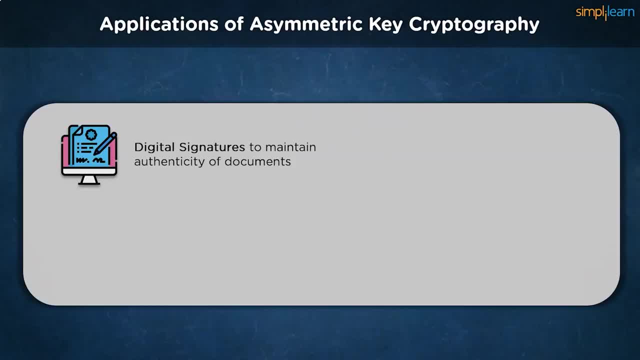 keys. Anyone who needs to verify the authenticity of such signatures can use the sender's public key to decrypt the signature. Since the public and the private keys are linked to each other mathematically, it's impossible to repeat this verification with duplicate keys. 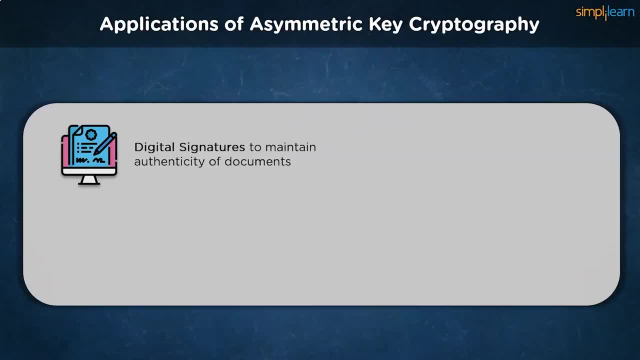 Document encryption has been made very simple by today's standards, but the background implementation follows a similar approach. In blockchain architecture, asymmetric key cryptography is useful. It is used to authorize transactions and maintain the system. Thanks to its two key structures, changes are reflected across the blockchain's peer-to-peer. 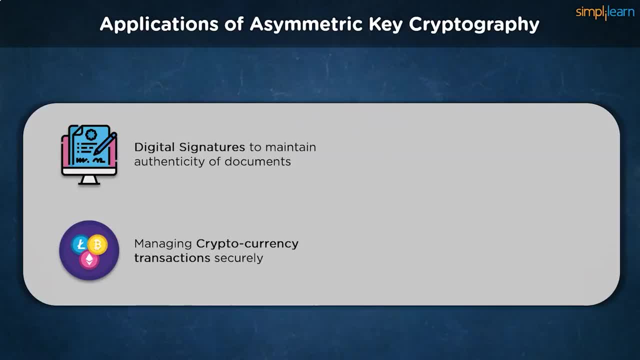 network only if it is approved from both ends. Along with asymmetric key cryptography's tamper-proof architecture, its non-repudiation characteristic also helps in keeping the network stable. We can also use asymmetric key cryptography combined with symmetric key cryptography to monitor SSL or TLS encrypted browsing sessions, to make sure nobody can steal our private. 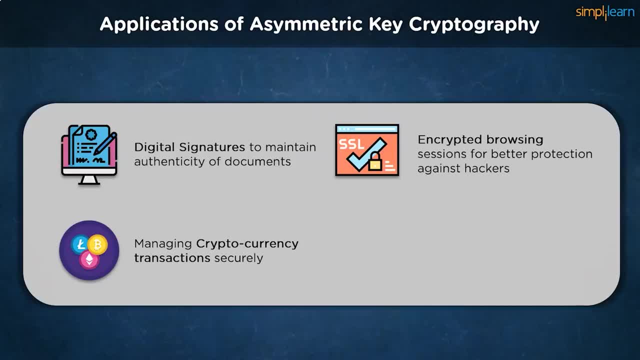 keys. Asymmetric key cryptography can be used to verify personal information when accessing banking websites or the internet in general. It plays a significant role in verifying website server authenticity, exchanging the necessary encryption keys required and generating a session using those keys to ensure maximum. 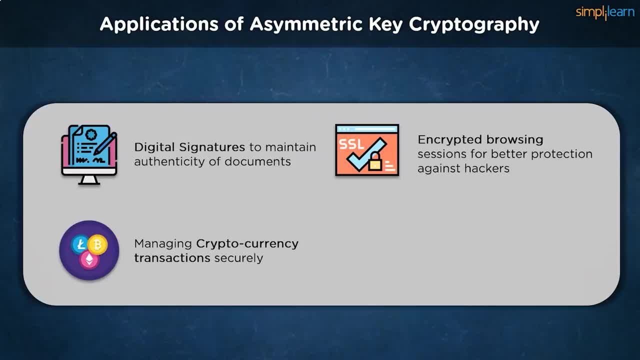 security instead of the rather insecure HTTP website format. Security parameters differ on a session-by-session basis, so the verification process is consistent and utterly essential to modern data security. Another great use of the asymmetric key cryptography is the use of the asymmetric key cryptography structure, which transmits keys for symmetric key cryptography. 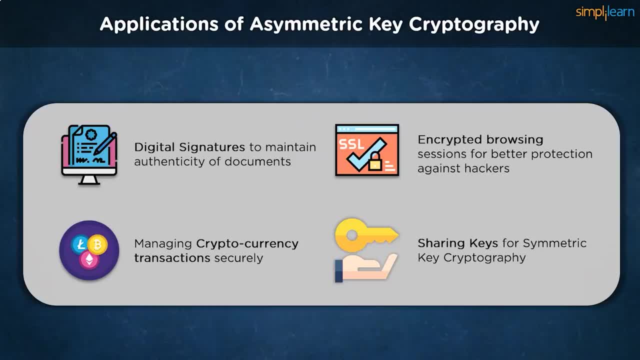 With the most significant difficulty in symmetric encryption being key exchange. asymmetric keys can help clear this shortcoming. The original message is first encrypted using a symmetric key. The key used for encrypting the data is then converted into the ciphertext using the receiver's public key. 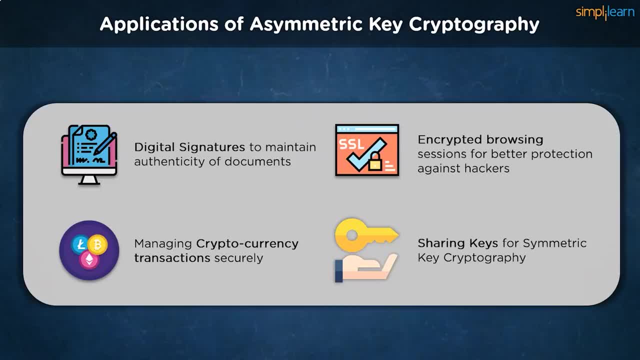 Now we have two ciphertexts to transmit to the receiver. On receiving both of them, the receiver uses his private key to decrypt the symmetric key. He can then use it to decrypt the original information on getting the key used to encrypt the data. 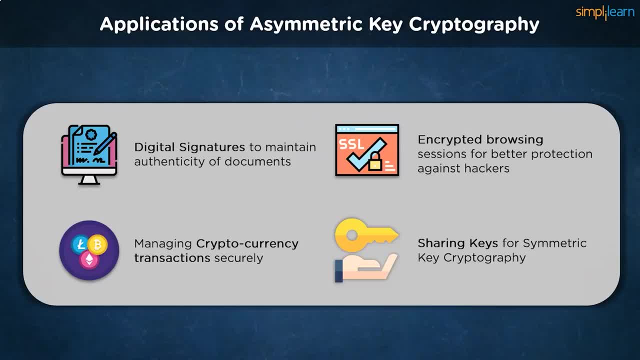 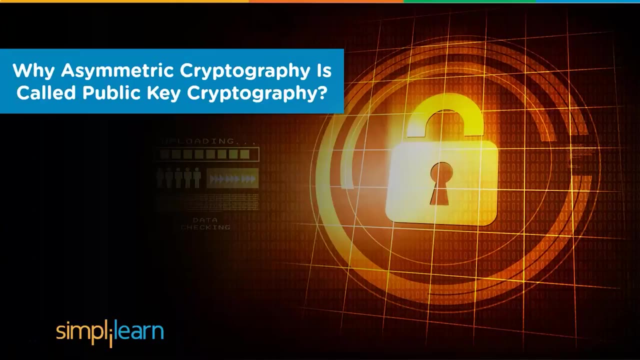 While this may seem more complicated than just asymmetric key cryptography alone, symmetric encryption algorithms are much more optimized for vast amounts of data. on some occasions, Encrypting the key using asymmetric algorithms will definitely be more memory efficient and secure. You might remember us discussing why symmetric encryption was called private key cryptography. 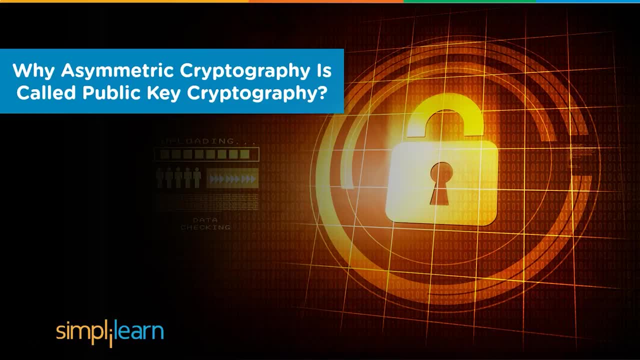 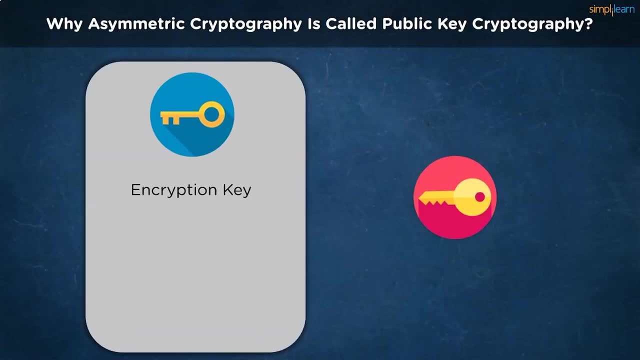 Let us understand why asymmetric encryption was called private key cryptography. Let us understand why asymmetric encryption was called private key cryptography. Let us understand why asymmetric falls under the public key cryptography. We have two keys at our disposal. The encryption key is available to everyone. 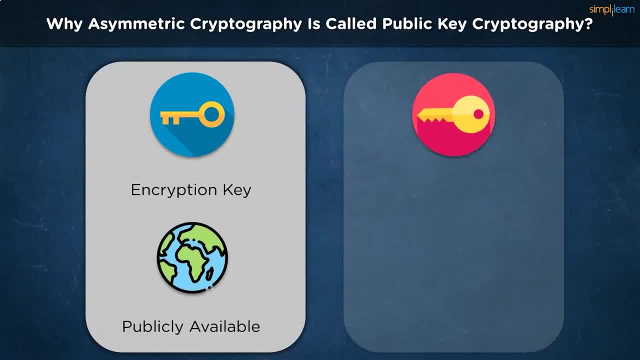 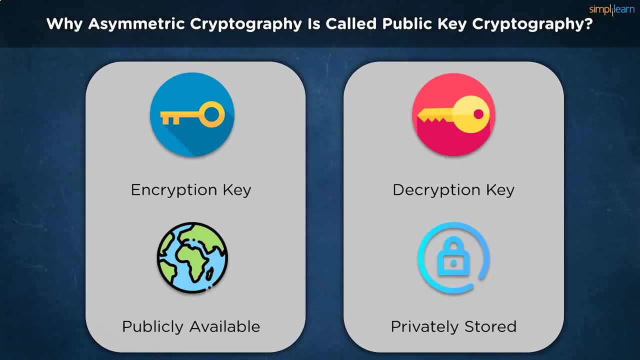 The decryption key is supposed to be private. Unlike symmetric key cryptography, there is no need to share anything privately to have an encrypted messaging system. To put that into perspective, we share our email address with anyone looking to communicate with us. It is supposed to be public by design, so that our email login credentials are private and 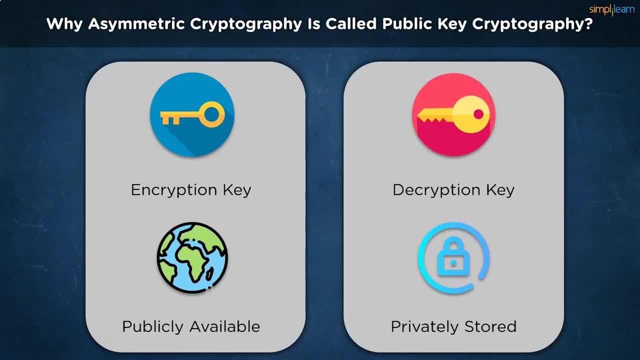 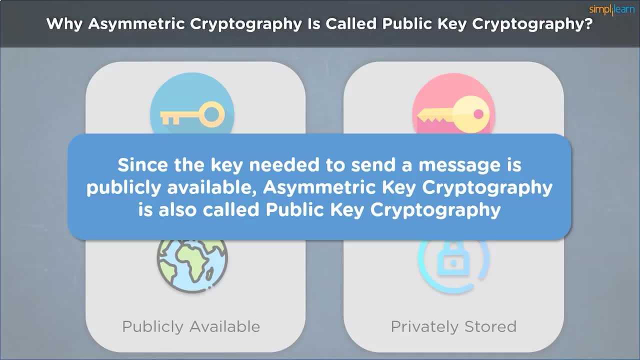 they help in preventing any data mishandling, Since there is nothing hidden from the world if they want to send us any encrypted information. this category is called the public key cryptography. There are quite a few algorithms being used today that follow the architecture of asymmetric 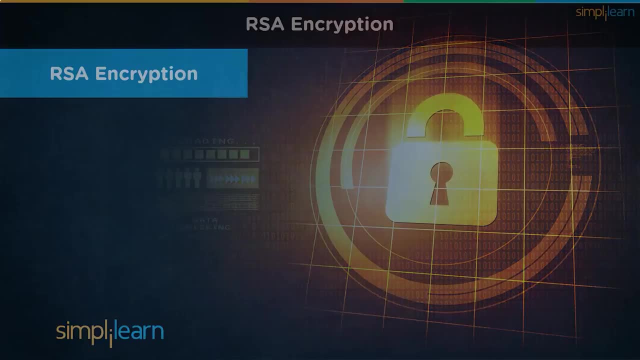 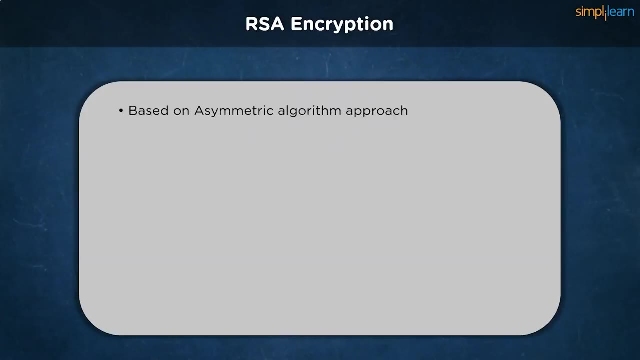 key cryptography none more famous than the RSA encryption. RSA encryption is the most widely used encryption or public key encryption standard using asymmetric key approach. RSA encryption is the most widely used encryption or public key encryption standard using asymmetric key approach After its founders Rivest, Shamir and Edelman. it uses block ciphers to obscure the information. 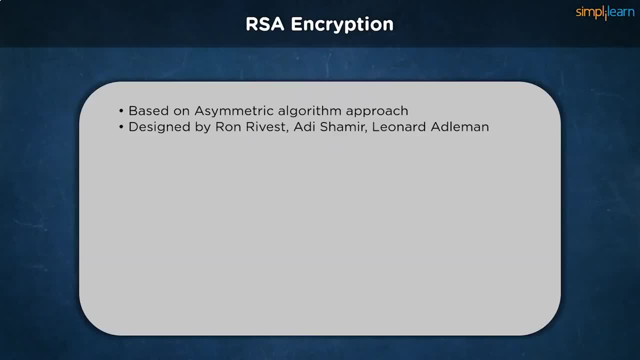 If you are unfamiliar with how block ciphers work. they are encryption algorithms that divide the original data into blocks of equal size. The block size depends on the exact cipher being used. Once they are broken down, these blocks are encrypted individually and later chained together. 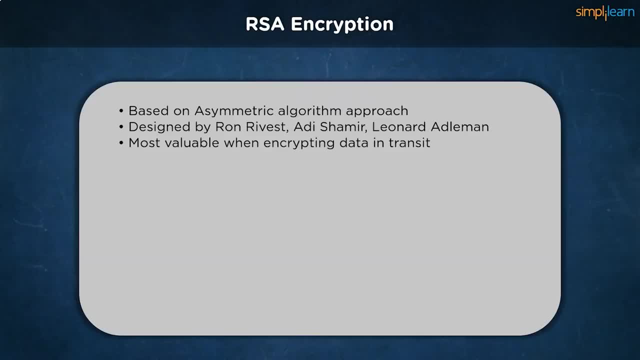 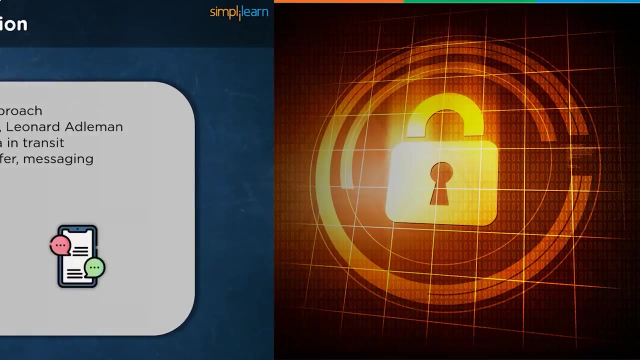 to form the final ciphertext. Widely considered to be the most secure form of encryption, albeit relatively slower than symmetric encryption algorithms, it is widely used in web browsing, secure identification, VPNs, emails and other chat applications. With so many variables in play, there must be some advantages that give.